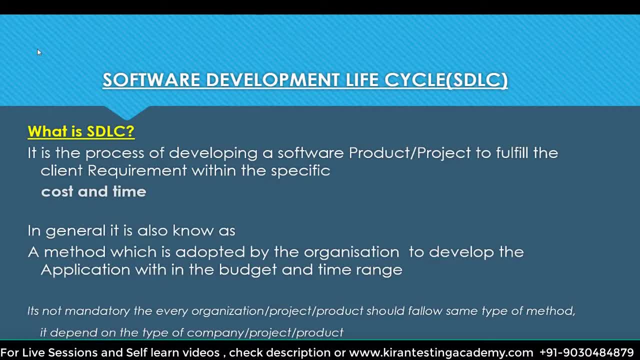 here. So what is SDLC? It's a process to develop an application or, in a simple words, I'll say it's a protocol or process or a guidelines to develop an application, right? So what happens if you follow the guidelines? What happens if you plan? Whenever you plan it? there are high chances that 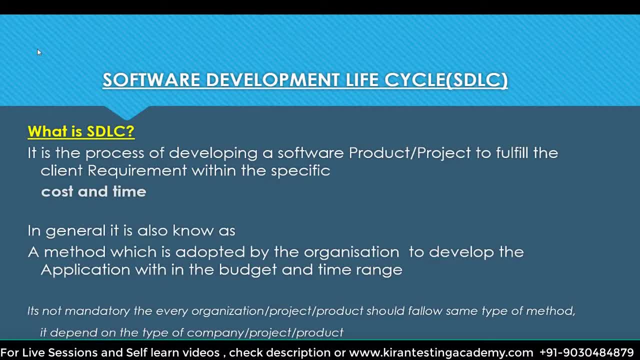 we can achieve our goal. What is our goal here? Our goal is to develop an application within given budget, right Within a given time frame and with quality. We can reach this whenever you plan it. Okay, so SDLC is planning. So if you are not going to planning and if you start working on that, 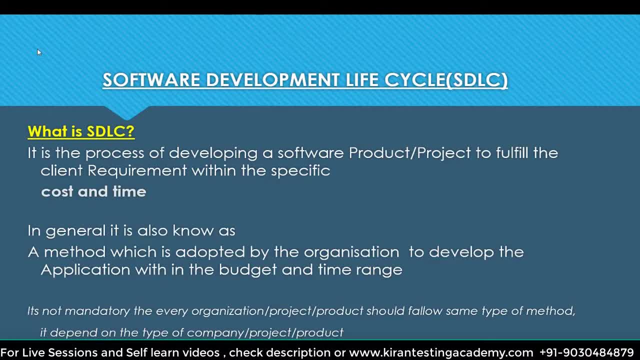 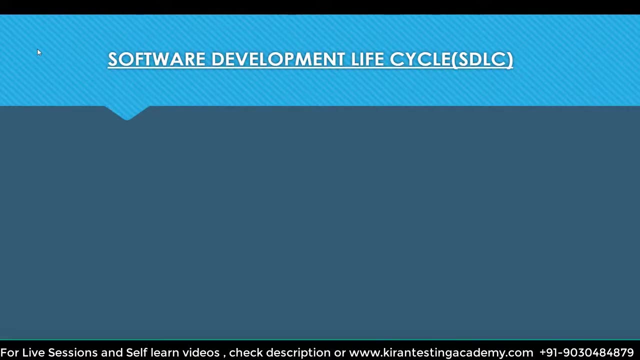 there are chances that you can drop somewhere in between, right? Yes, a proper planning will give you excellent result, will take you to your goal, right? Yes, that is what SDLC is. Now let's move on to the phases of SDLC. These are the common phases of SDLC. 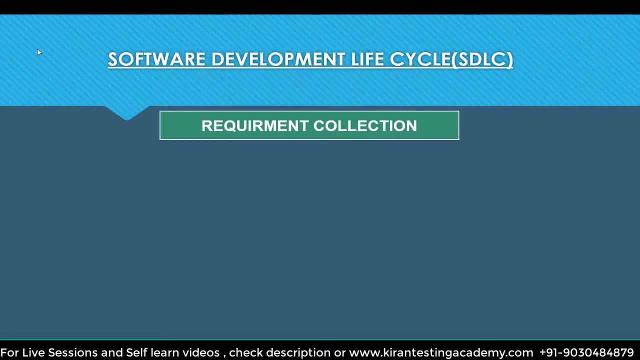 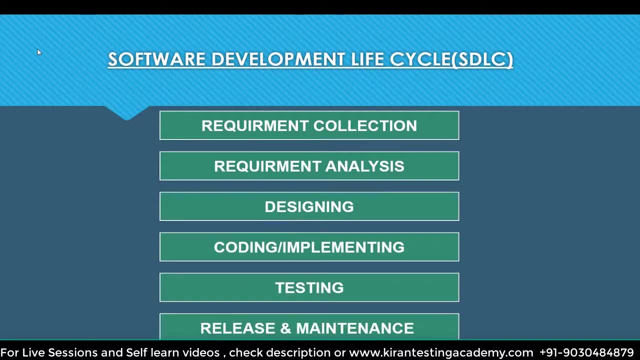 Here we can have a look on this: Requirement collection analysis, designing, coding, testing, release and maintenance. These are six phases of your software development lifecycle. Okay, in some cases you can see requirement collection analysis combined as requirements only. Okay, release and maintenance are two different phases. Okay, yes, Now let me explain. 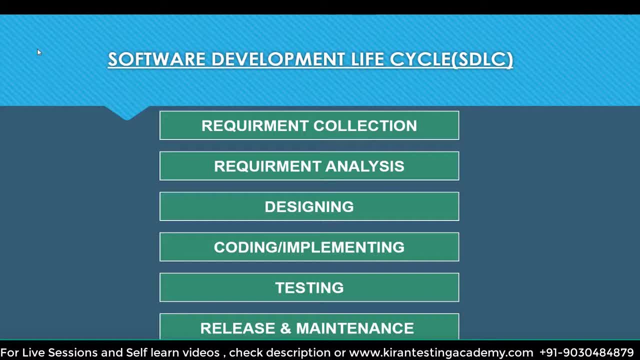 you this: How to develop an application. So SDLC is a process to develop an application, How exactly the software development lifecycle works. Okay, so what we do is we'll talk theoretically and also we are going to talk about what happens in an organization level. So here we are going. 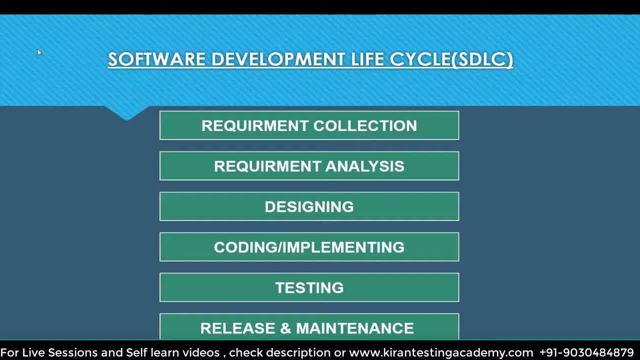 to talk about what happens in each phase. Okay, what documents will be released in each phase and how those documents are useful for testers. Okay, you may have hundreds of documents in the complete development lifecycle, but all documents are not useful for the tester right. Yes, 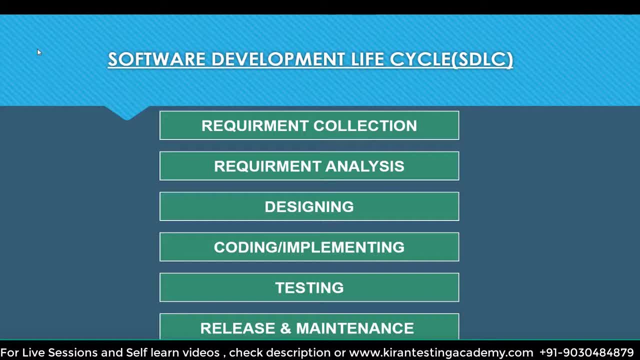 some documents are more useful for the tester. What are those and how to go through those documents, All those details we are going to have a look on. Okay, so let's begin with the very first phase, that is, requirement collection, As the name indicates. okay, collecting the requirement from the client. Who will collect? 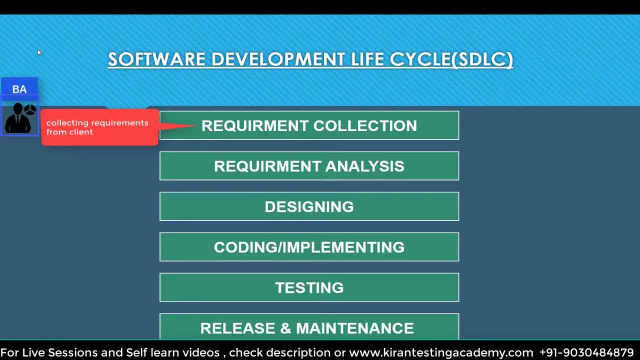 the requirements generally: BA business analyst. He's going to interact with the client. Okay, he is going to have multiple meetings with the client and he is going to take all his requirements. Whatever the client says, he is going to write in a documentation and that. 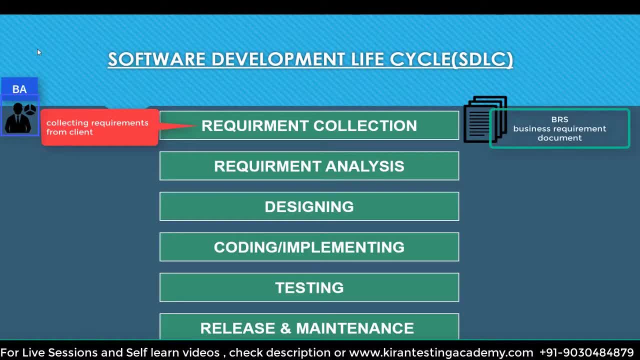 name of the documentation is business requirement specification, or BRD, what we call it, as It has all the business needs. Okay, only requirements, right? Fine, So next phase. after taking the requirement from the client, we'll move on to the next phase. Okay, in. 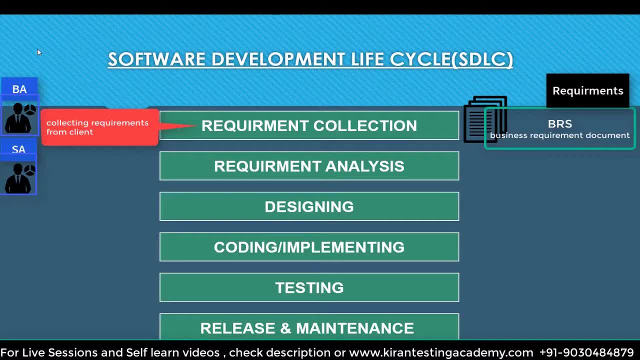 this phase, system analysts will participate along with business analysts. He is going to interact with the client, Okay, and what the system analyst is going to do is he is going to develop the functionalities for the requirements. Okay, as discussed in the first phase, we got the requirements right For the requirements functionalities. 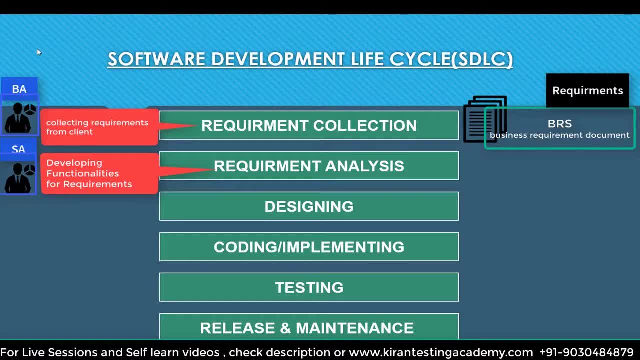 will be defined in this phase, the requirement analysis phase, and all the functionalities will be defined in a document called functional requirement specification document or system requirement specification document. We call it as FRS or FRD. Okay, here see all these. 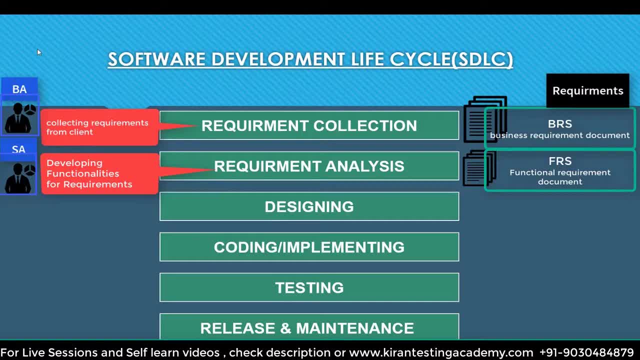 are. standards means requirements should be taken by BA. This is a standard right. Assume that we have a small company where we have three or four employees over there, Then there is no concept of BA right. A senior developer or CEO or someone will take So that information. 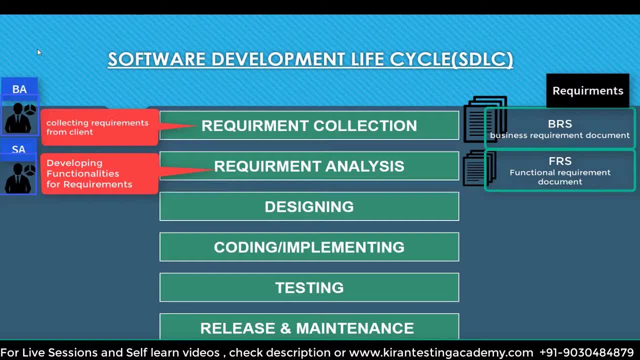 what I am giving you. this is just a standard. Lot of companies will follow this, Some may follow it, but some companies may not follow it due to their own reasons. Clear Yep Now. so next we are going to move on design phase. So in this phase, design architect. 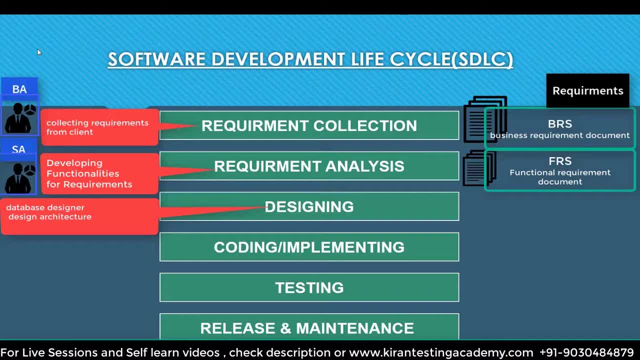 database designers will participate. Depending on the requirement documentation, depending on the BRS and FRS documentation, they are going to develop the design. First graphical user interface design document will be given. Database design documents will be produced. Okay, So these documents will be produced in this High level and low level documentation for. 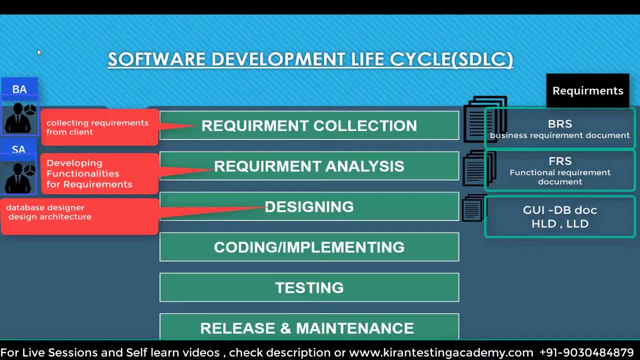 the developers. Okay, Those documents will be produced in the design phase. Next it will move on to the coding phase. Your developers will code the application depending on the information given. Then, after it will move on to the testing phase, Tester will perform. 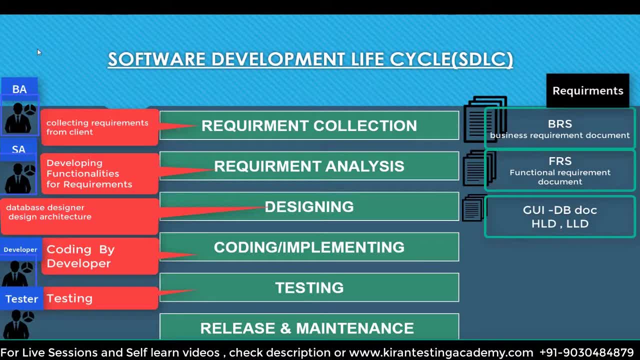 end to end testing on the application. If everything is fine, we are going to release that to the client. After releasing whatever the change you are going to have to do, you changes you want to make. that falls under maintenance. okay, this is an walkthrough of your. 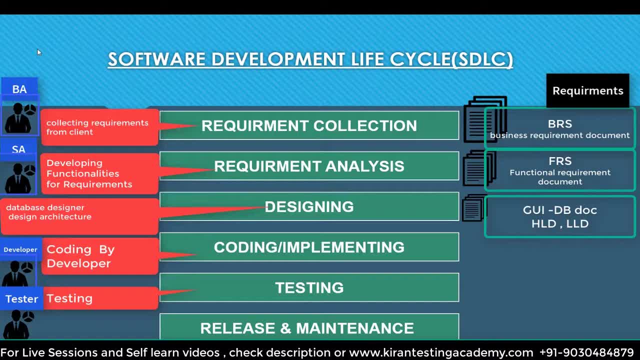 software development life cycle. okay, here, two or three major things: what we need to discuss. the very first major thing what we need to discuss is, sorry, in the first phase, what i said: your ba take the requirement from the client and he is going to put the document called brs and this: 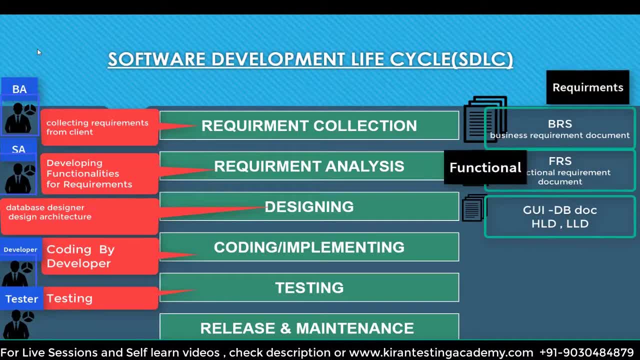 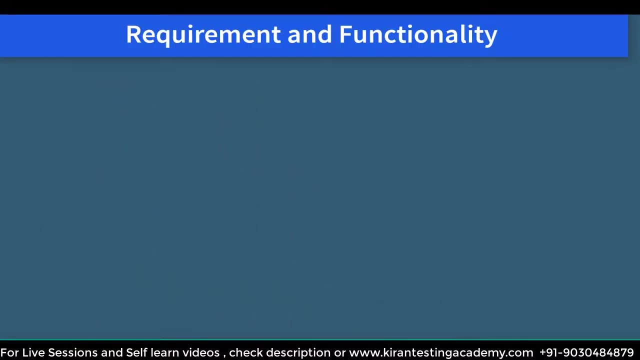 is a requirement related document. right in the second phase the requirements will be converted into functionalities. so what is the difference between requirement and functionality? just think and let me know. yes, there is a vast difference between functionality and a requirement. see, in the brs document we have only requirement. what client want in a simple line, in a 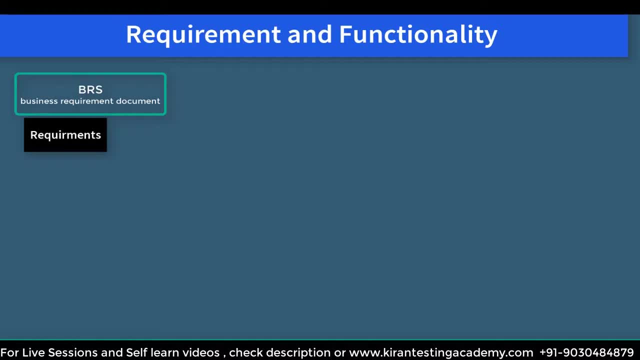 single line. that's it. okay, assume that i have a banking application. client is giving a requirement for the banking application. client said that my client should have a option to transfer money from one account to other account. we call this as bank to bank transfer. okay, so bank to bank. 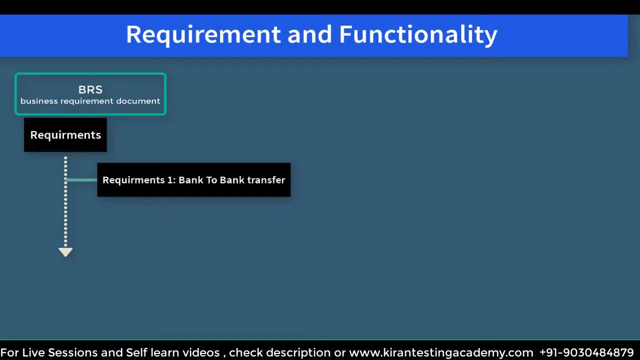 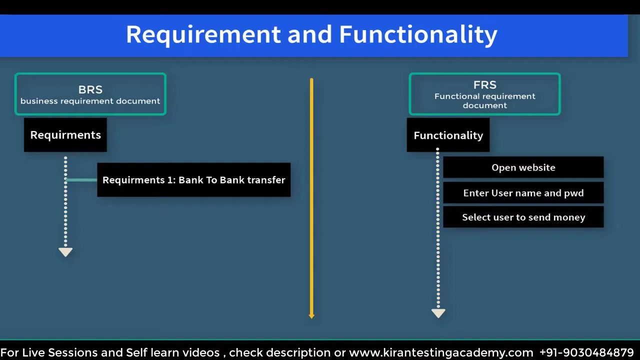 transfer should be available. right. bank to bank transfer should be available for the users. this is a client requirement. okay, so what is the functionality of it? yes, open the website. enter username and password. okay, select the user to whom you want to send the money. if user is not available, add that user. okay, enter how much money you want to send. enter high. 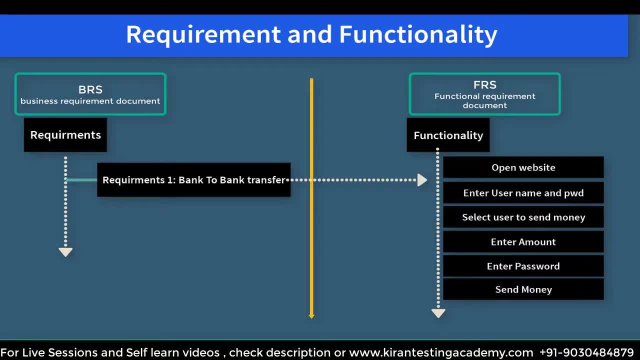 security password. click on send. this is the functionality for this requirement. okay, this is difference between the functionality and requirement. so what is very important here? yes, functionalities plays a very important role, so frs document plays a very important role. you need to read, understand that frs document clear. next, one more thing: actually taking the 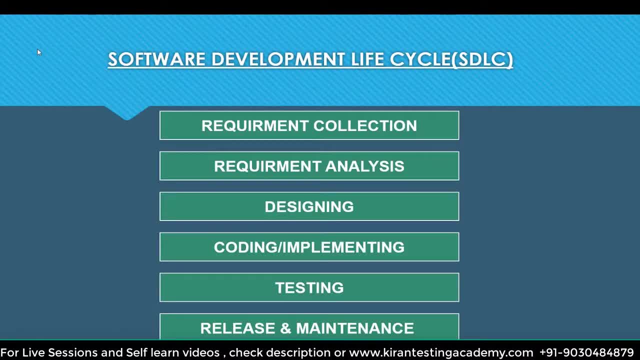 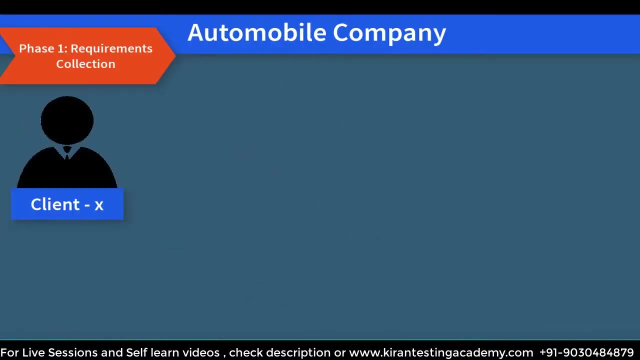 requirement doesn't mean that we have started a project. yes, that's true. assume that let's come out of this software development and we'll talk about a generalized topic here. see, i have a automobile company. a client x has approached me and he is giving his requirements. my ba is taking down the requirements. 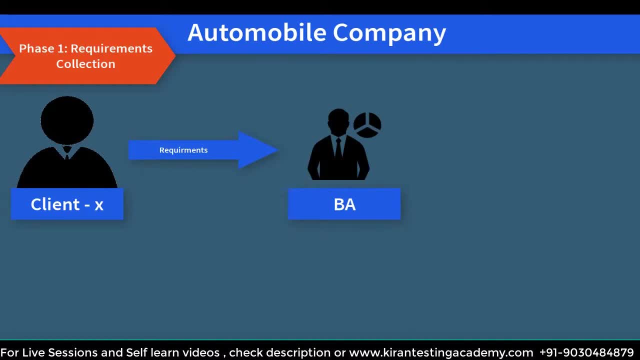 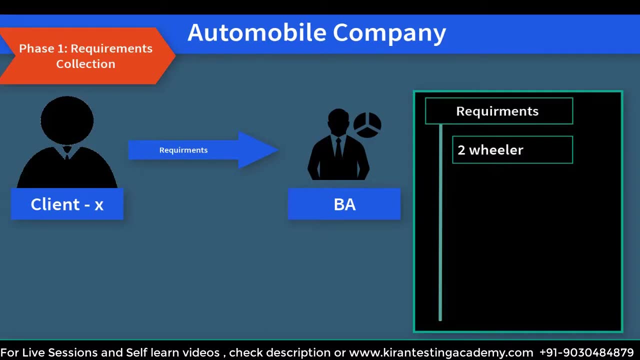 of the client. okay, so client requirements are something like this: he want a two-wheeler. next, it should give mileage of 30 kilometers per liter, it should run at the speed of 100 kilometers per hour, which should be three seating capacity, which should be in black in color, which should run with diesel. these are the requirements given to 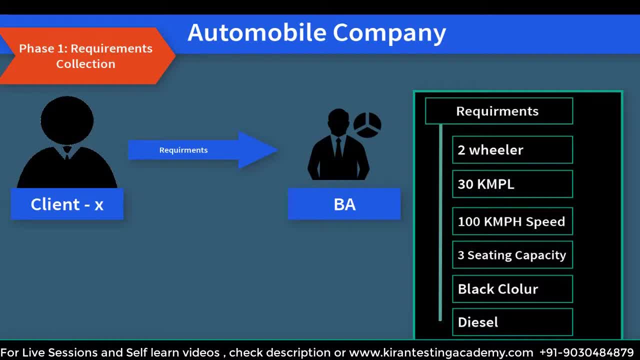 my ba. okay, yes, my ba has taken all the requirements of what we do next. so we are going to take a wrench and start working. no, right, we are going to analysis each and every part: whether we can do it or not, whether it is realistic or not, whether it is feasible or not. yes, so here we are going to. 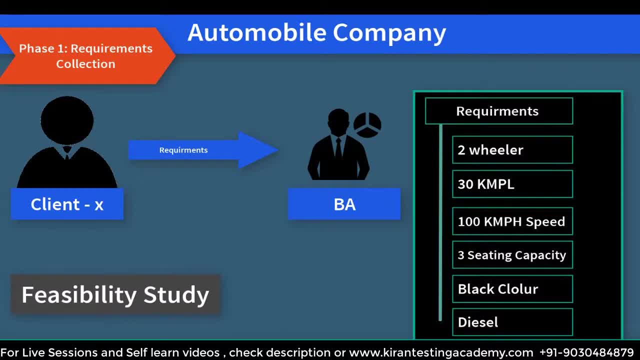 conduct a study called feasibility study, to check whether it is feasible or not. yes, so here we are going to study: the given requirements are really realistic or not, whether we can fulfill it or not. two wheeler: yes, we can produce. okay, with 100 kilometers per hour. yes, we can do it, we should. 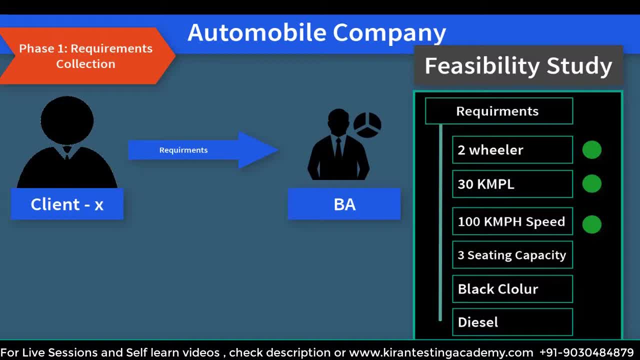 give a mileage of 30 kilometers per liter. yes, we can do it. three seating, a two-wheeler with the three seating is against the law, right? so we'll study like step by step, then we'll report it to the client saying that guys, three-seater is not possible. if you want to go. 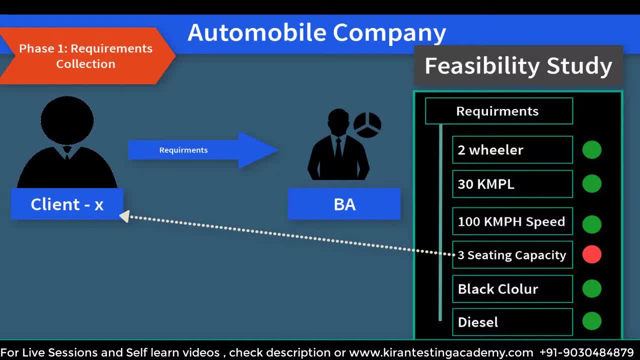 with two-seater, okay. if client says that no, no, i want three-seater- signal, normally negotiations will start okay. so we'll do it with two-seater, okay. client says that: no, i want three-seater at any cost. we'll close that. as dlc over there. project is closed. the same applies for software. 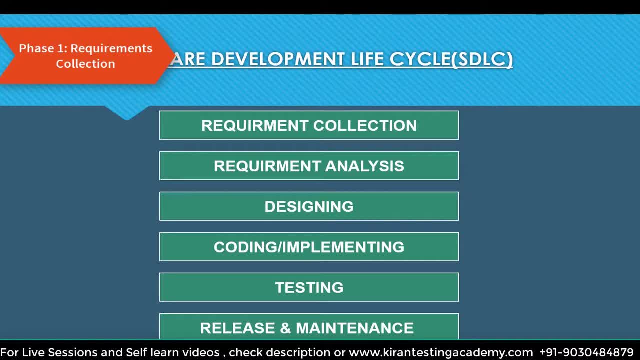 also, we have taken the requirement from the client. it doesn't mean that project is standard, right? client gives you, client gives us- a hell lot of requirements, right? yes, we need to check that whether it's realistic or not what we are going to do in the feasibility study. yes, 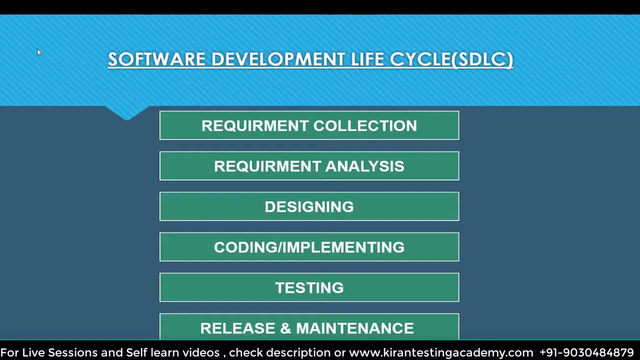 we are going to check the technology budget, whatnot everything. client said that, guys, i want a selenium testers. or client said that my application should test with selenium. now, we'll check that whether we have selenium testers or not, right? so if you have converts, a manual to. 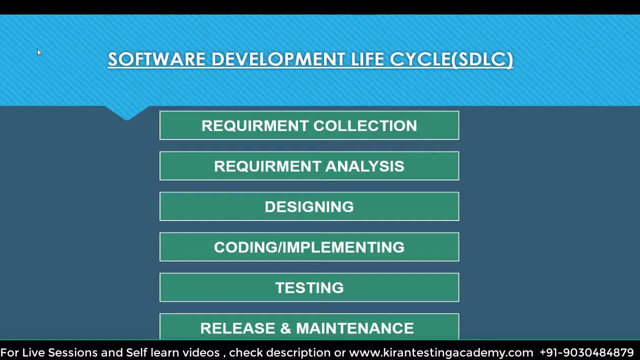 selenium will it work or not, whether it comes in a budget or not, right? yes, not only that client said that: okay, i want so and so technology. we'll see that, whether the technology is available or not, whether we can do it or not. so all these factors will be discussed in a study called feasibility study, if it passes. 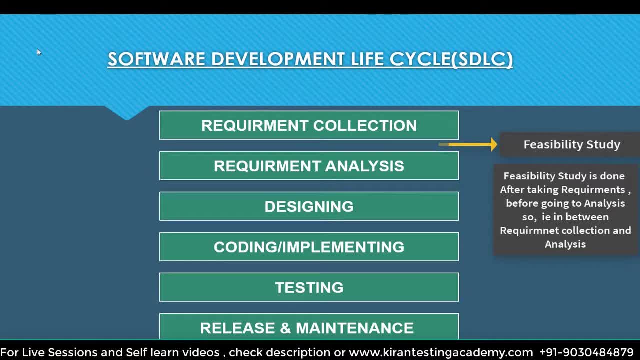 the feasibility study, then only it will go to the next phase, like requirement analysis phase, else it will not move on to the next phase. as simple as that, clear. so this plays a very, very, very important role. feasibility study plays a very, very, very important role. yes, because this is a decision factor. why? because see client. so who will do this? 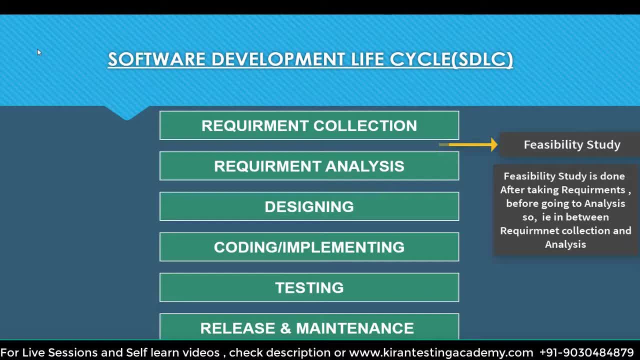 feasibility study generally. BA should do it. business analyst is the one who will do this study study. but as it's a important one in some companies, there will be a group of people who discuss about that. okay, a group of people will sit and they are going to discuss about. 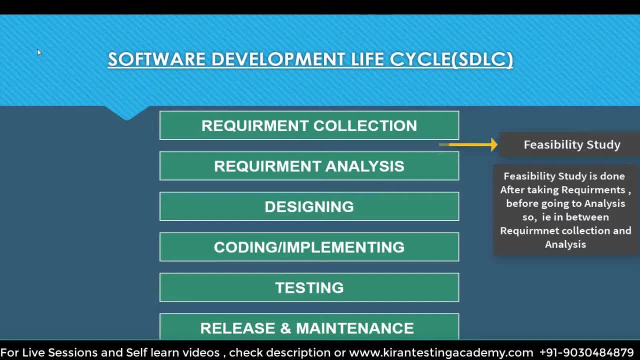 requirements. if they like senior developers, like senior members from different environments, they will sit and they will discuss on the requirement. okay, once, once, if it is fast with the past, with the feasibility study, then it will move on to the next phase or actually the project is started.